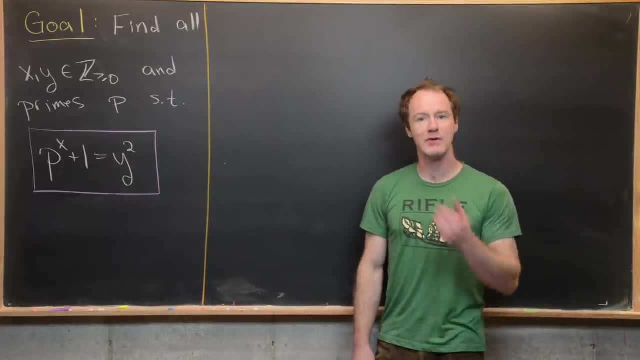 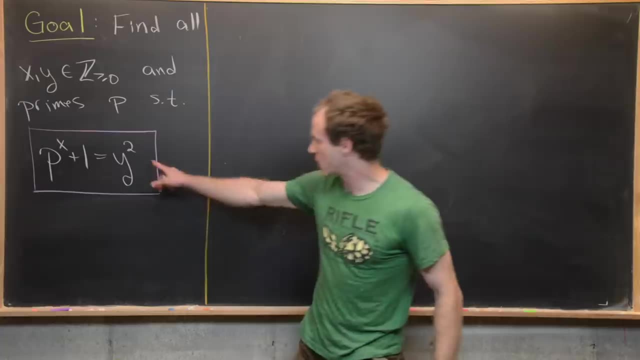 squared. So I'm not going to give any hints or anything, but maybe, if you want to try this problem, go ahead and pause the video and give it a go. Okay, so now let's jump into the solution. So the fact that we have y? squared on one side of the equation and plus one on the other side of the 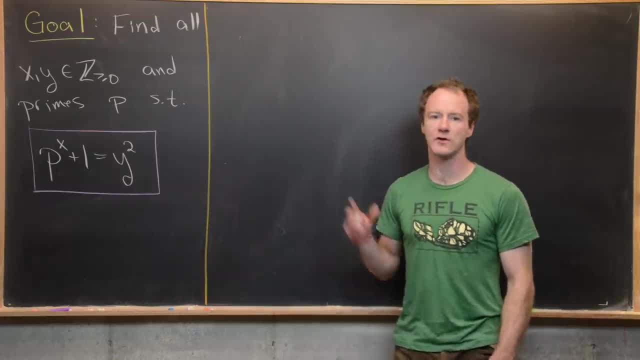 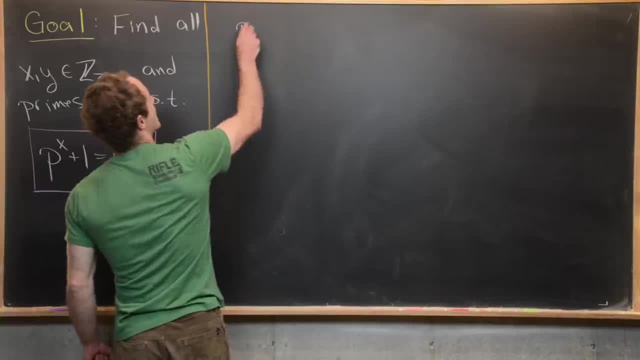 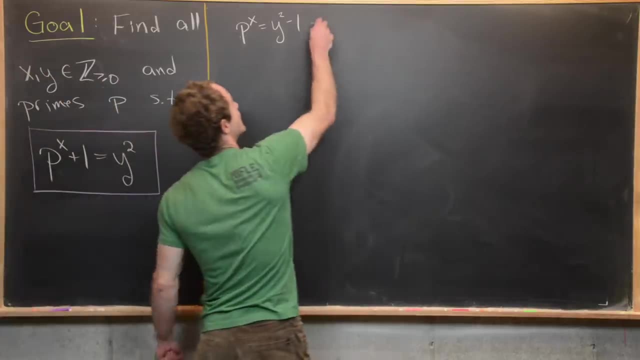 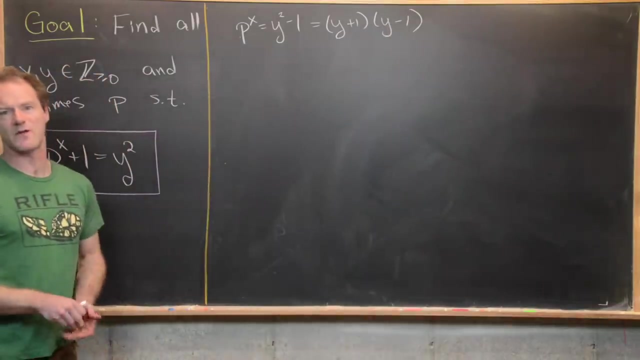 So let's do that, So let's do that, So let's start by doing that. So we're going to write p to the x equals y squared minus one, and then factor this thing on the right hand side to y plus one times y minus one. And now we want to make the following obvious but very important observation: 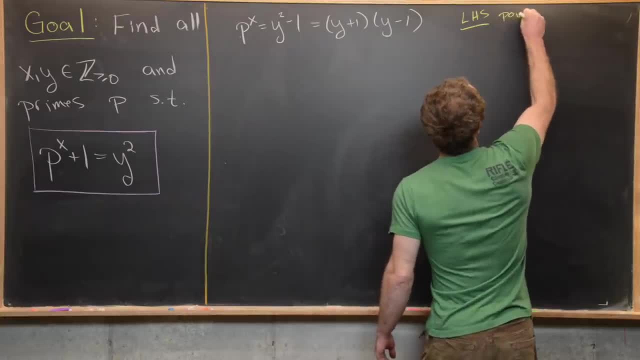 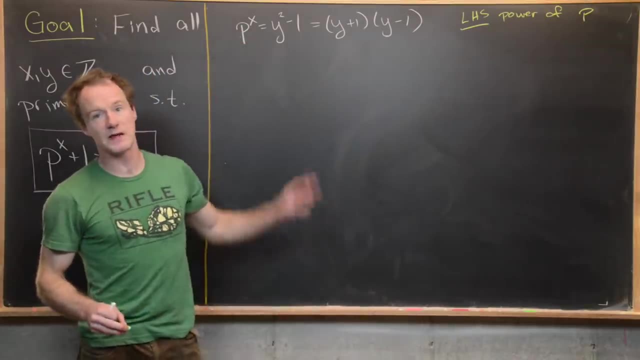 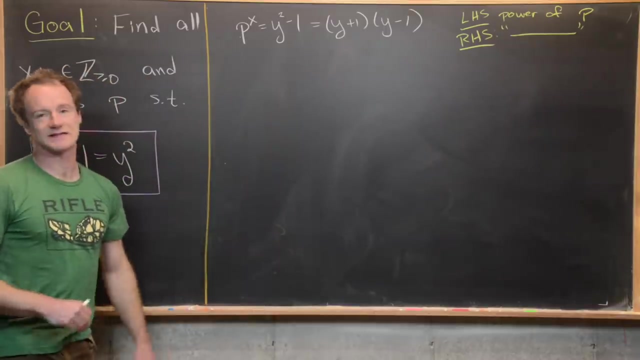 and that is the left hand side, is a power of a prime p. But if the left hand side of the equation is a power of p, then also the right hand side is a power of p. But the fact that the right hand side is a power of p and we have factored it into two parts- 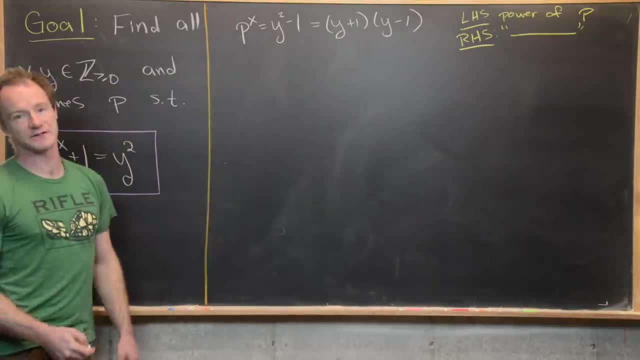 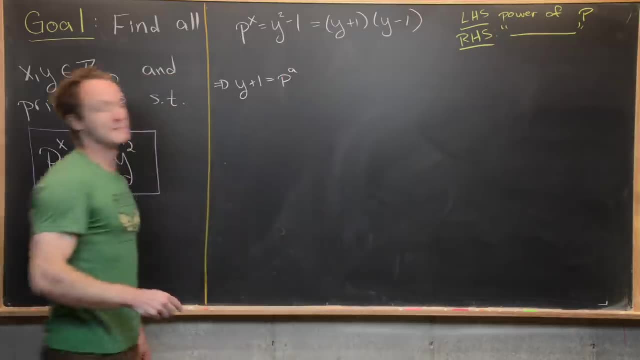 that means each of these parts is a power of this prime. So that means we have the following fact: We have: y plus one equals p to the a for some a. and then we have y minus one is equal to p to the b for some b. 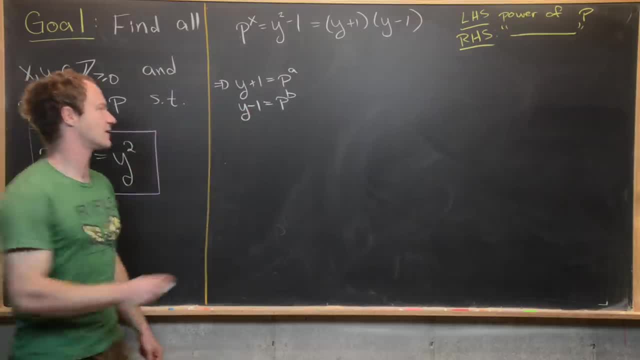 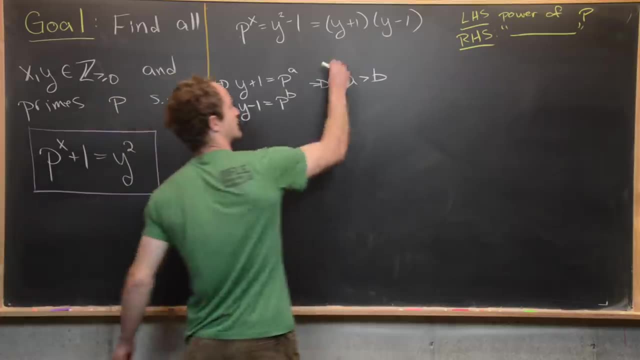 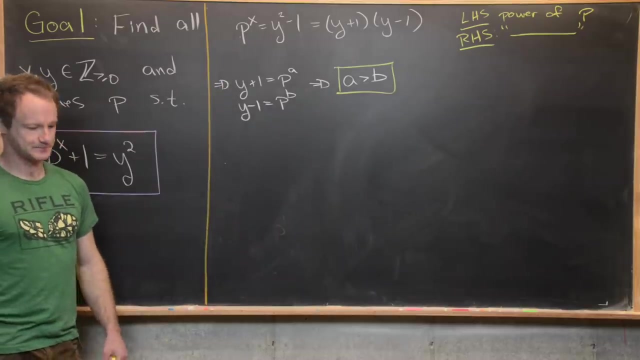 And then also, since y plus one is bigger than y minus one, that trickles down to the fact that a is bigger than b. So that's an important thing to notice and that'll get us started with the next step. Now we want to look at this system of equations and notice if we could reduce this. so we only 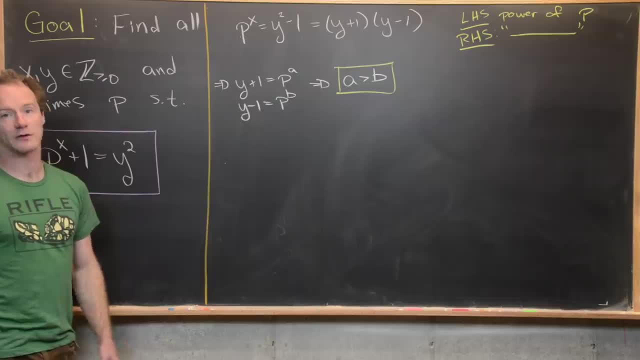 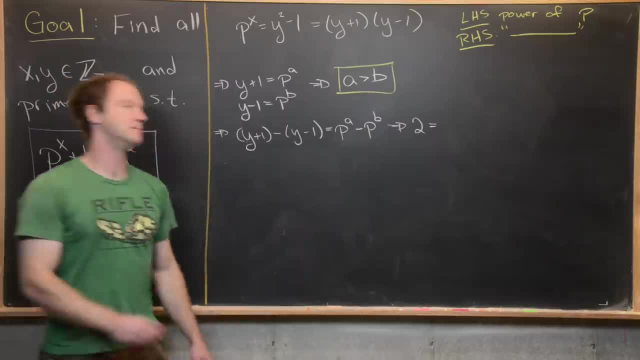 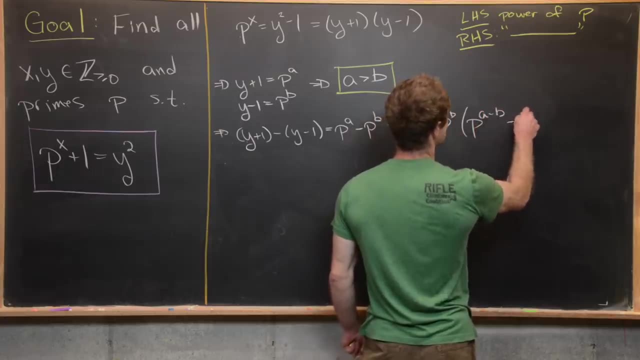 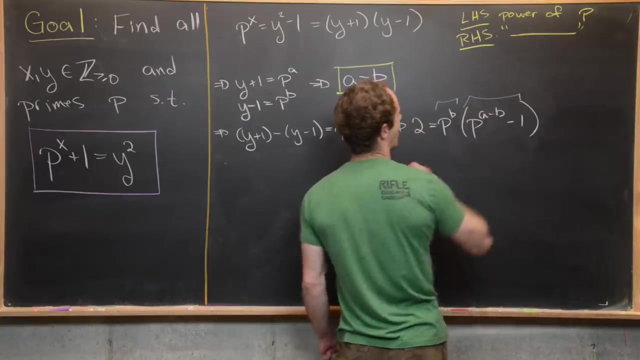 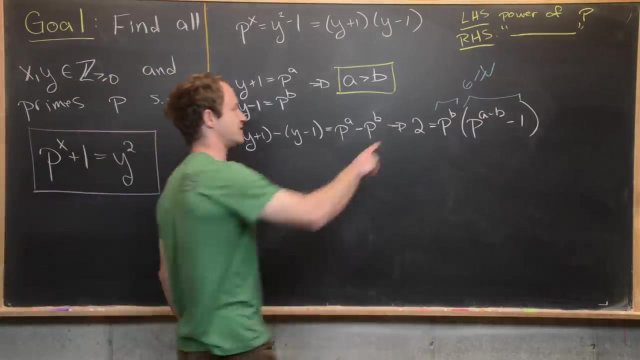 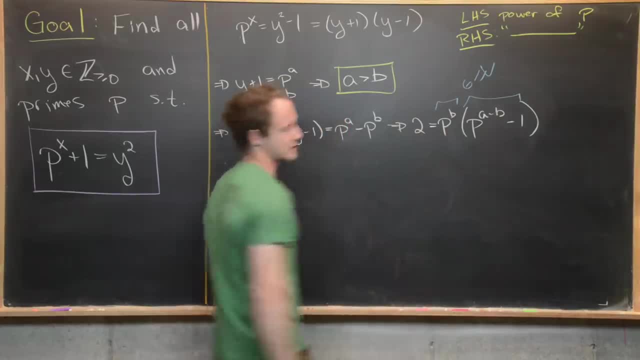 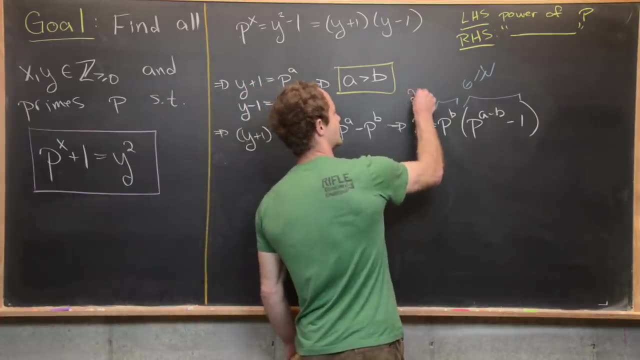 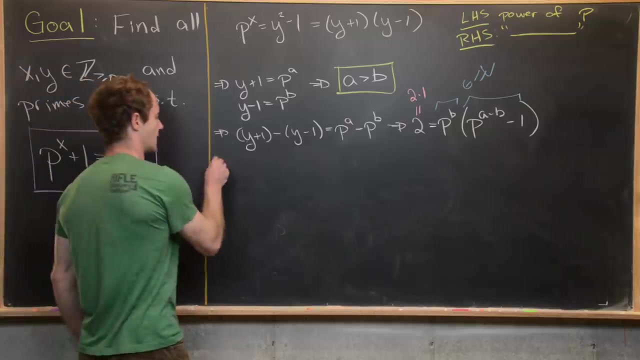 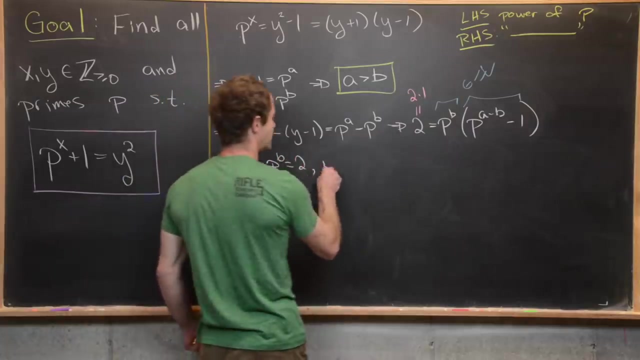 that means one of these is equal to one and the other is equal to two, But that breaks into two cases based off of those two choices. So just to reiterate, we're using the fact that the only way to factor two into a product of two natural numbers is as two times one. Okay, so let's look at our first case. So our first case will be: p to the b equals two, and then p to the a minus b minus one equals one. So that's our 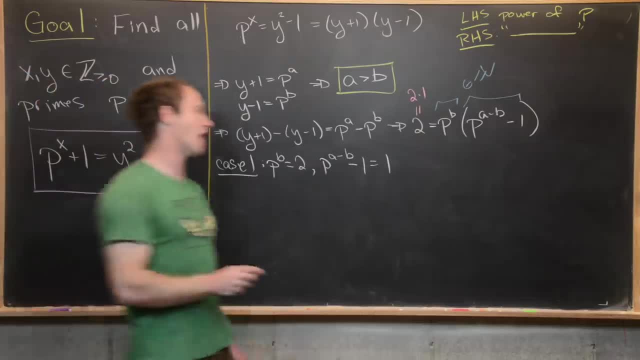 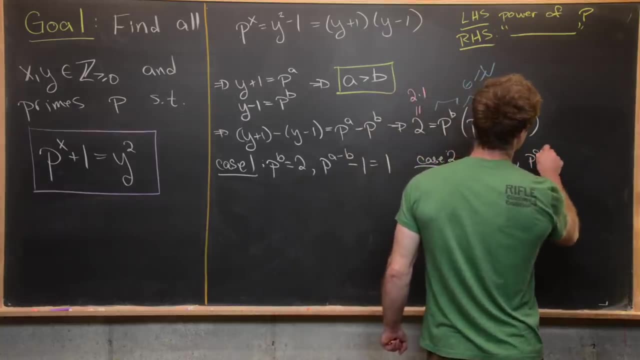 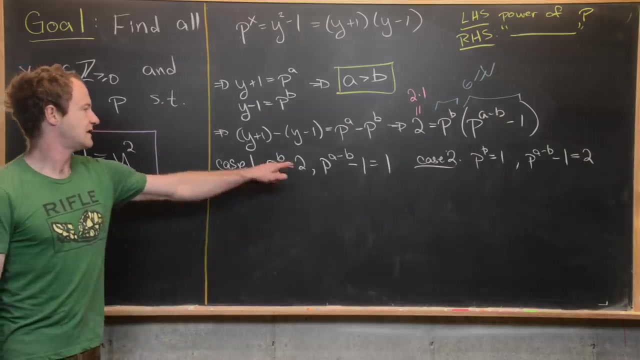 first case, And then we can split up that factorization of two the other way, And that'll give us our second case, which is: p to the b is equal to one, and p to the a minus b minus one is equal to two. So let's see what this first case gives us. Well, if p to the b is equal to two, 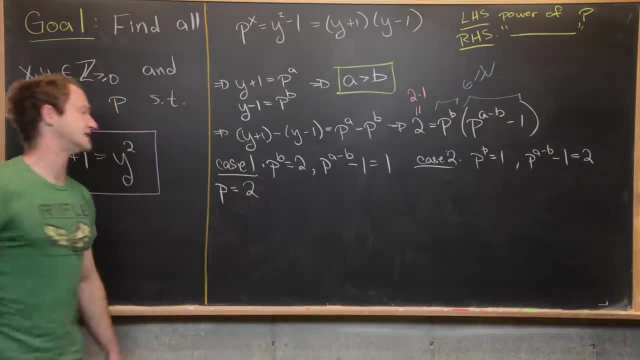 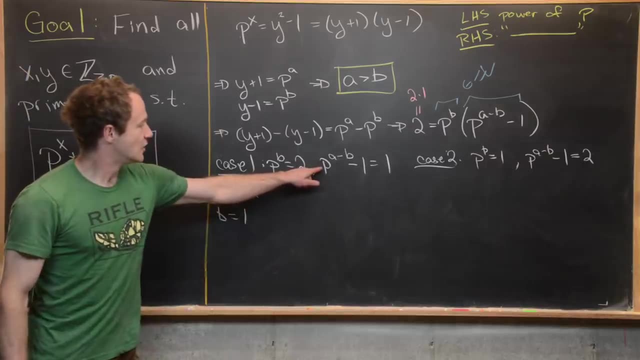 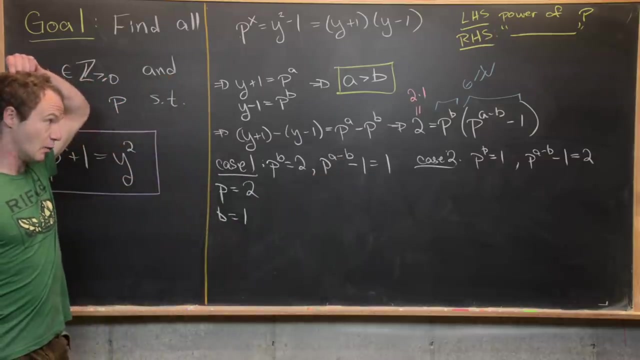 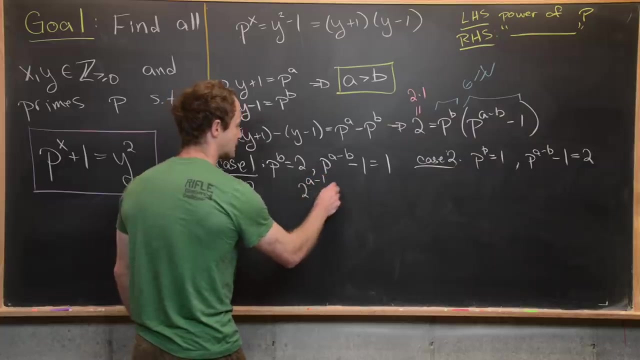 well, that means immediately that the prime p is equal to two and the number b is equal to one, like that. Then next we can reduce this to two to the a minus b equals two by adding one to both sides of the equation, But then we know b is equal to one. So this is really two to the a minus one. 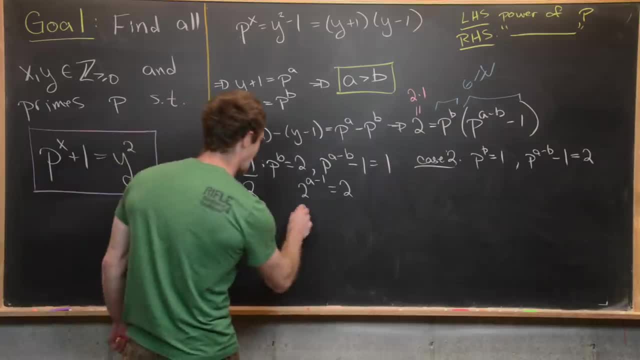 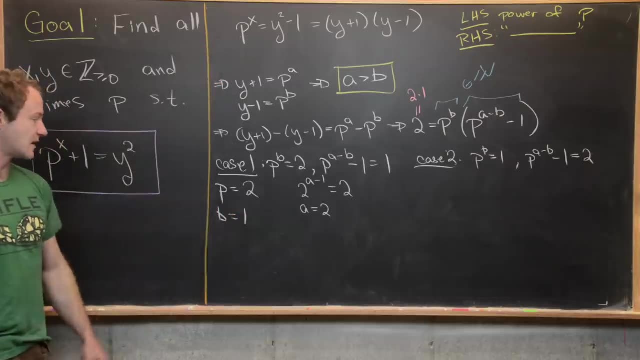 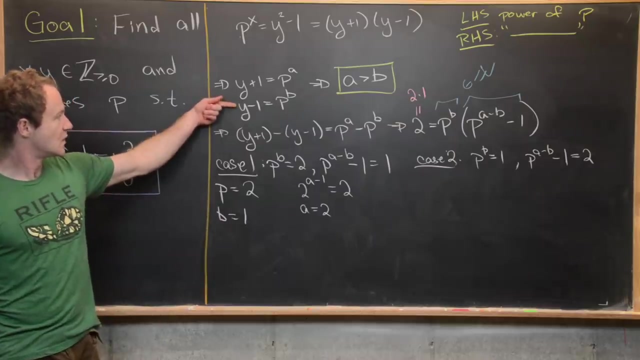 equals two, But that tells us that a is equal to two. Now we can insert these parts into our equations up here and that'll give us y pretty quickly. So maybe we'll insert this b into this equation. We'll see that y minus one is equal to two to. 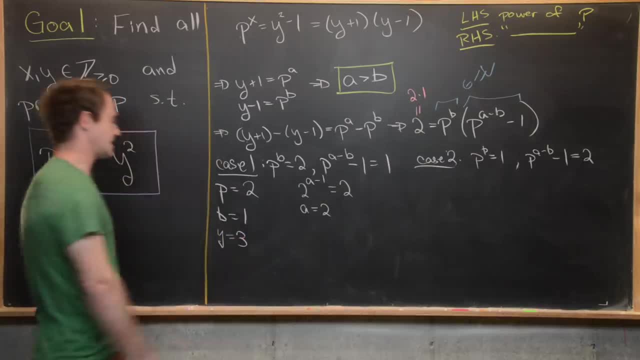 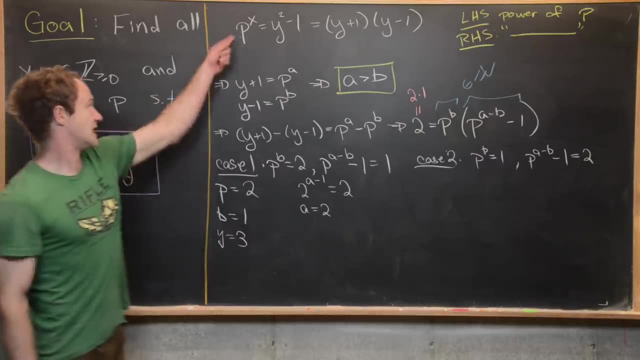 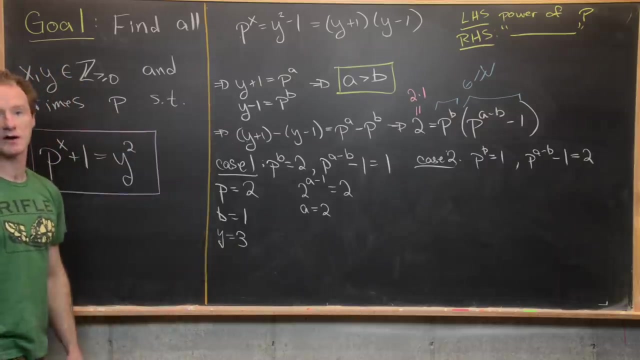 the one, But that means y is equal to three. But then, finally, we can stick this value of y into our original equation, either here or here, And we'll see that two to the x is equal to three squared minus one. But if two to the x is equal to three squared minus one, 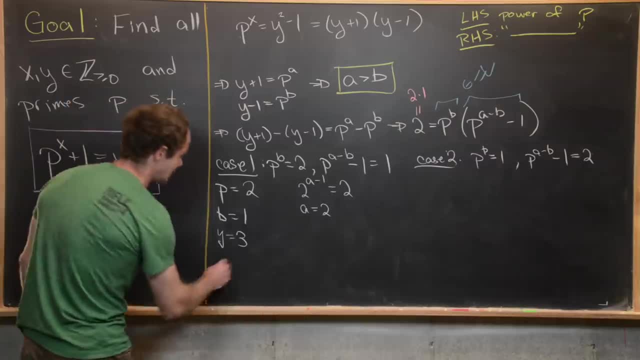 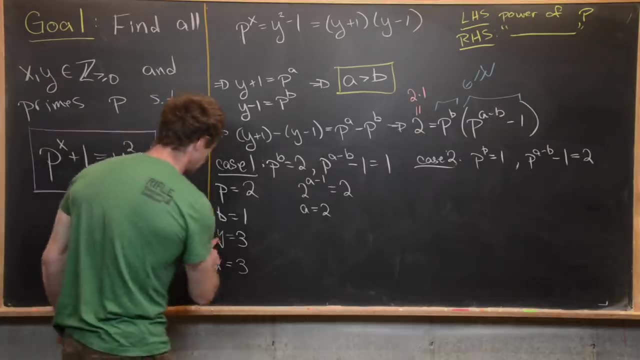 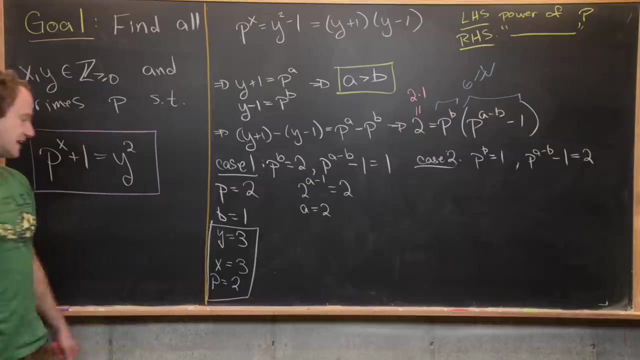 one, that's the same thing as 2, to the X equals 8, which means X equals 3. so there, we've got our first solution. so Y is equal to 3, X is equal to 3 and then P is equal to 2, so I'll just put that right there. so they're next together, okay, so